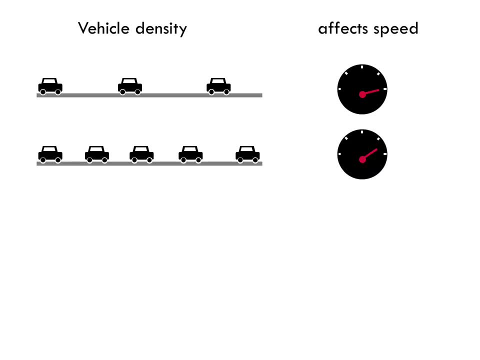 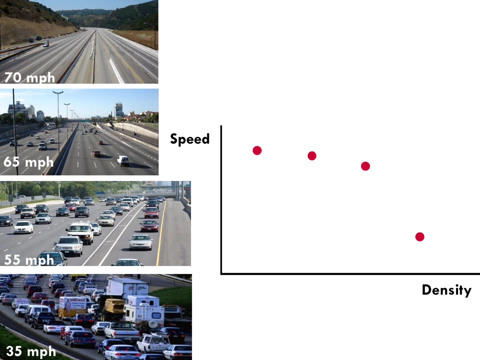 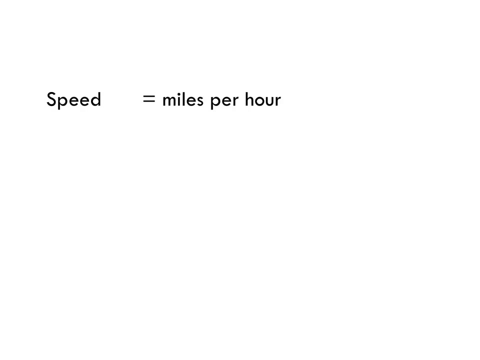 drivers can travel quite fast, But as we add cars, drivers must slow down. Here's what that looks like graphically: As we add cars to the roadway, drivers must slow down. You'll notice that this is a non-linear relationship. So we've talked about speed, which is pretty intuitive, and we've talked about vehicle. 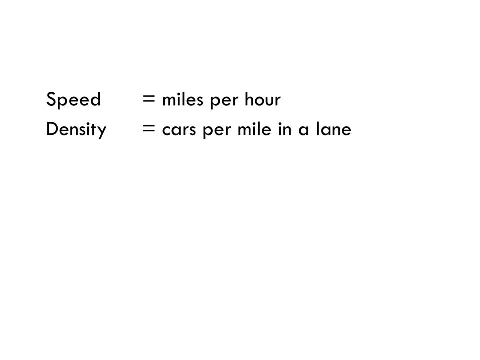 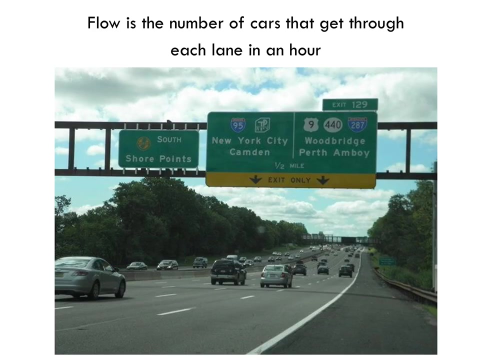 density. the number of cars per mile in a lane. Traffic flow is density times speed or the number of cars per hour passing a point on a roadway. You can think of flow as the number of cars who pass under this sign each hour. 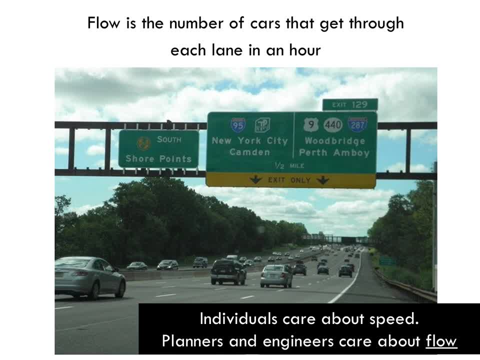 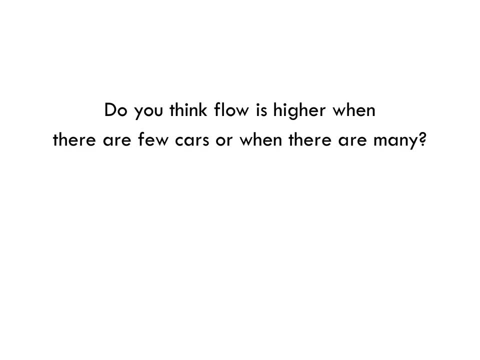 Individuals care about speed Planners and engineers they care about flow. Do you think flow is higher when there are few cars or when there are many? It's not fair. It's a trick question because it totally depends. Let's take a look. 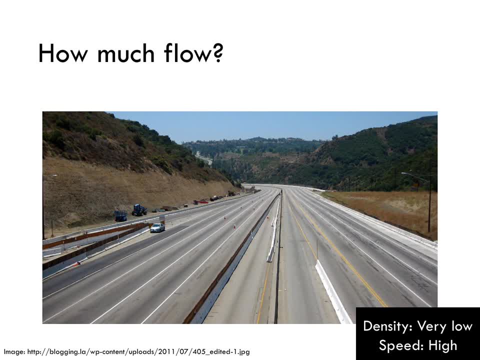 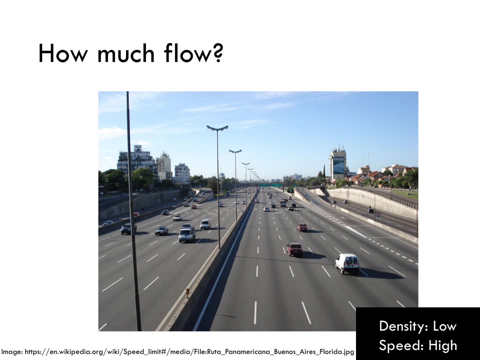 This is the 405 during Carmageddon. In this photo the 405 has very low density and someone could drive very fast, But flow is pretty low. Here we still have pretty low density and drivers are still able to maintain a high speed. 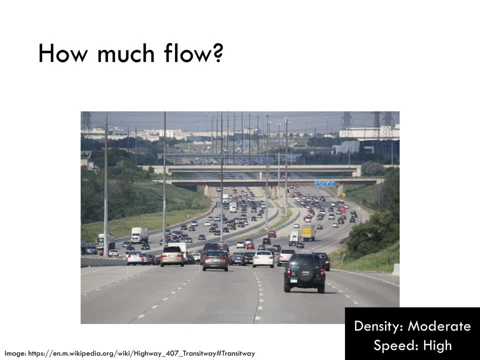 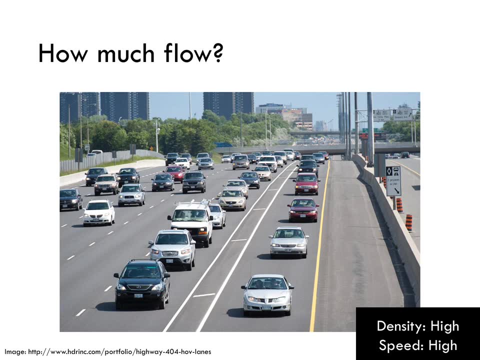 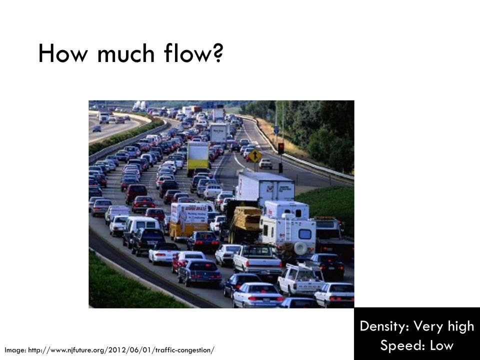 Here flow is higher still. Here density is high and speeds are high. Which lane do you think has the highest flow In this photo? density is so high drivers have to slow down to a crawl. Flow here is very low. I want you to take a moment to think. 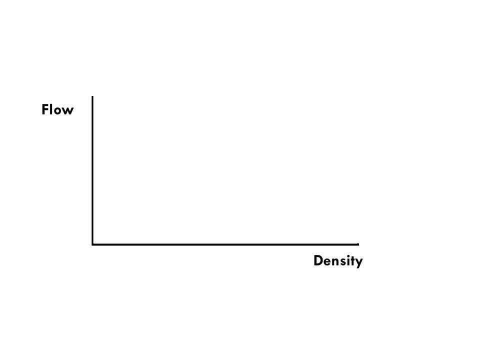 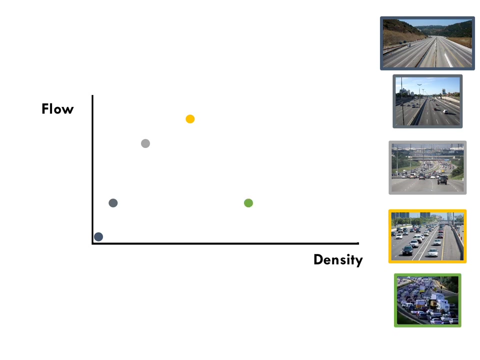 about the relationship between flow and density. Try to graph out each of the points we've seen so far. Here's what that looks like: Low density and low flow in the lower left corner, and as we move to the right we increase density and increase flow up until a point and then adding more cars. 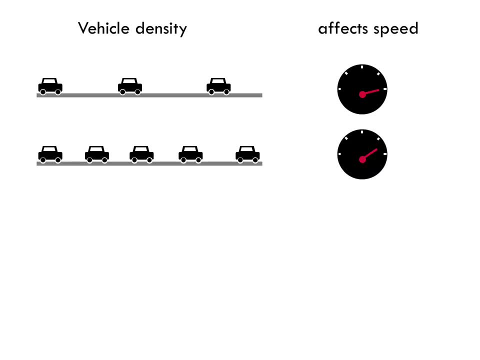 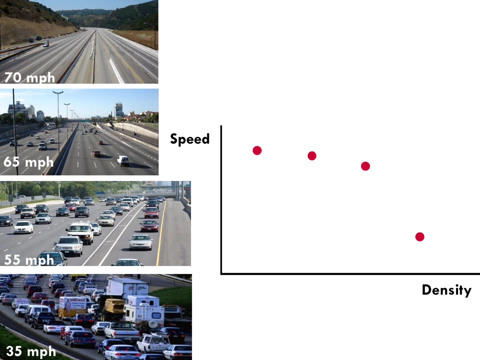 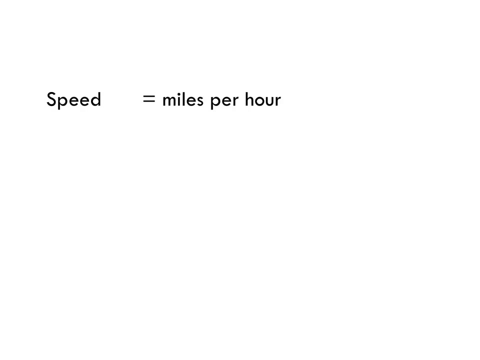 drivers can travel quite fast, But as we add cars, drivers must slow down. Here's what that looks like graphically: As we add cars to the roadway, drivers must slow down. You'll notice that this is a non-linear relationship. So we've talked about speed, which is pretty intuitive, and we've talked about vehicle. 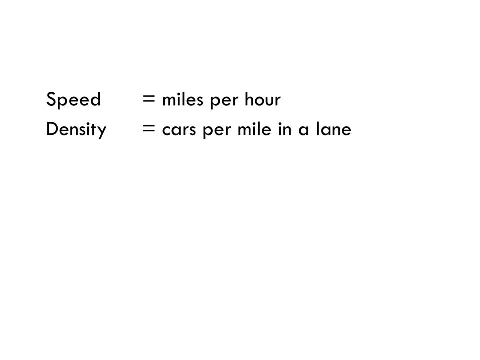 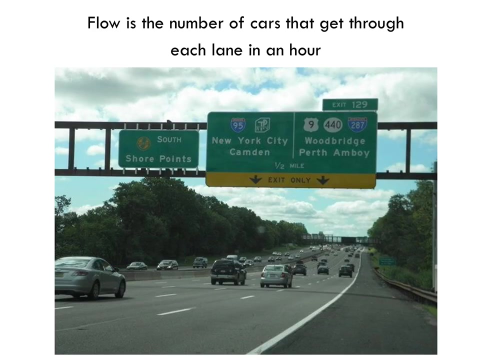 density. the number of cars per mile in a lane. Traffic flow is density times speed or the number of cars per hour passing a point on a roadway. You can think of flow as the number of cars who pass under this sign each hour. 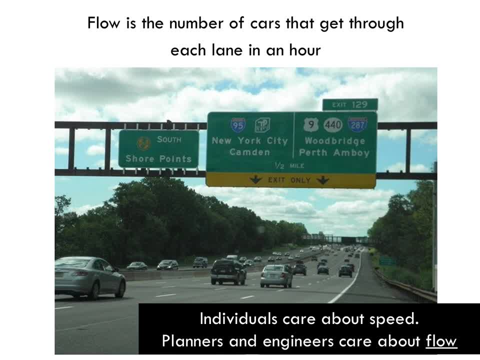 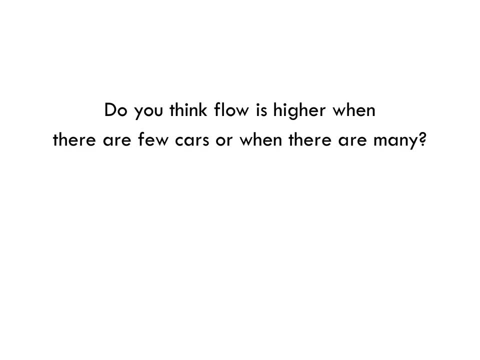 Individuals care about speed Planners and engineers they care about flow. Do you think flow is higher when there are few cars or when there are many? It's not fair. It's a trick question because it totally depends. Let's take a look. 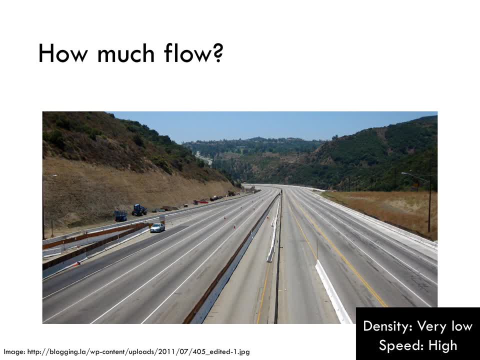 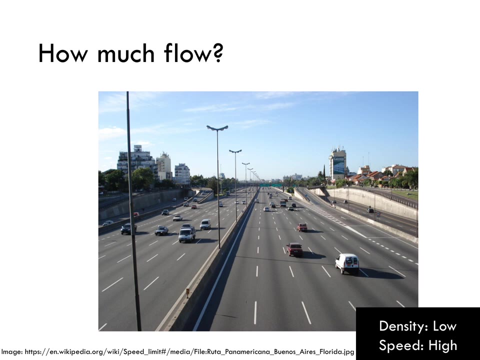 This is the 405 during Carmageddon. In this photo the 405 has very low density and someone could drive very fast, but flow is pretty low. Here we still have pretty low density and drivers are still able to maintain a high speed. 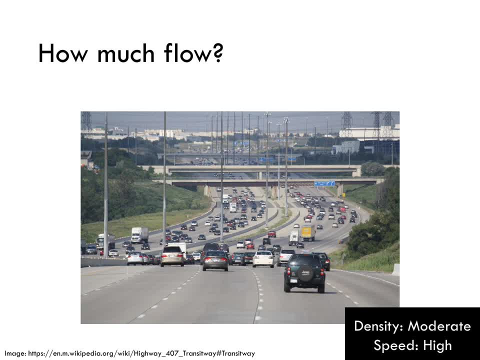 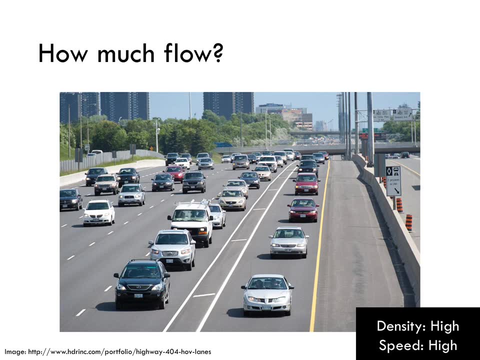 Here flow is higher still. Here density is high and speeds are high. Which lane do you think has the highest flow? In this photo, density is so high that drivers have to lie at a place calledorsa to explain. Here density is high and speeds are high. Which lane do you think has the highest flow? 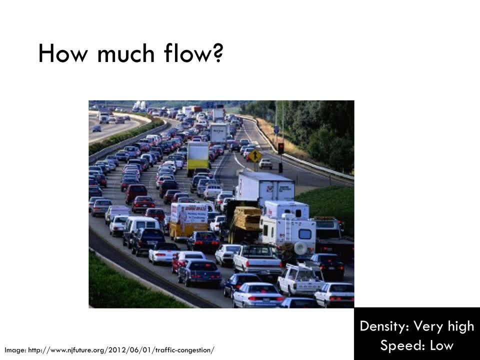 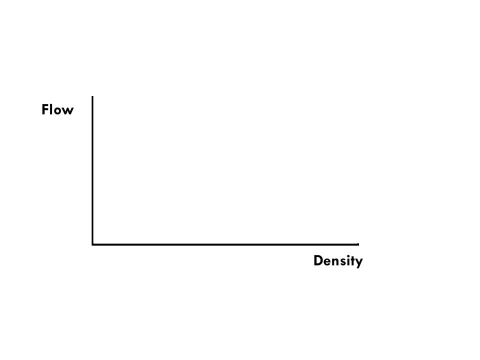 to slow down to a crawl. Flow here is very low. I want you to take a moment to think about the relationship between flow and density. Try to graph out each of the points we've seen so far. Here's what that looks like: Low density and low flow in the lower left corner.